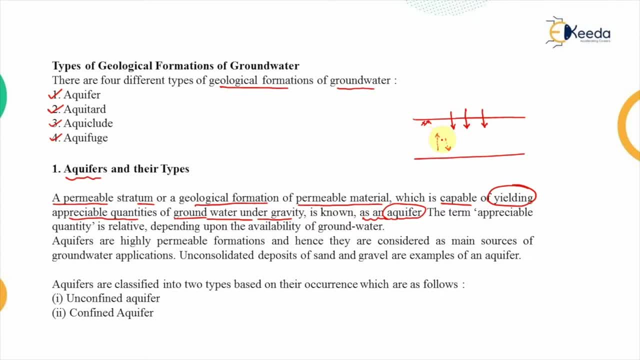 we can also extract the water. Such formations are known as the aquifer, Now here the term that is appreciable quantity. that is a relative term because that depends upon the availability of the ground water. If the water table is very high, then obviously the water which can be extracted that will also be very high. 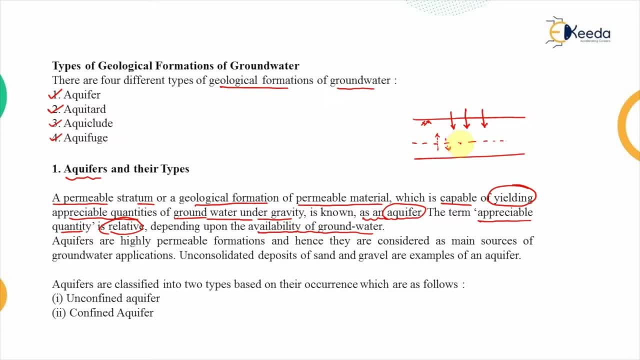 But if the opposite is true, then there will be lesser quantity, There will be lesser quantity of water which will be available. So aquifers are highly permeable formations because permeability and porosity- we have studied these two parameters which define whether we would be able to extract the water or not. 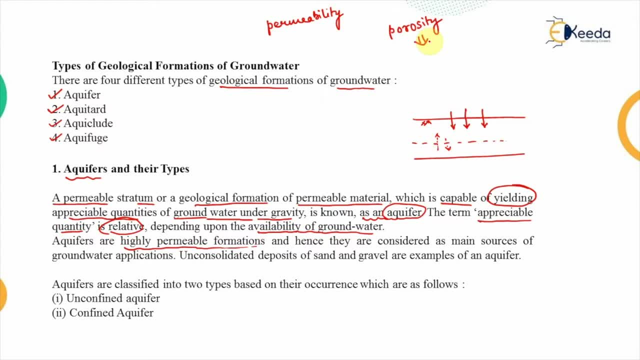 So the porosity that tells us whether the water is stored within the rocks or not. So will water be stored In the rocks that is identified with the help of porosity? If a formation is porous, that means the water can be stored in them. 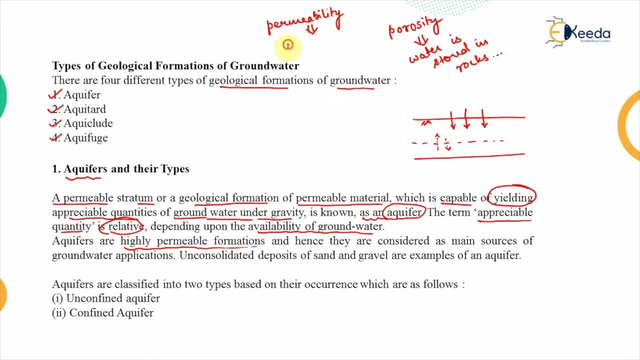 And if a strata is permeable, that means water can be extracted from them. So to have the extraction on the ground water, it is pertinent to have the structure as permeable as possible And since aquifers are highly permeable, they are considered as the main source of the ground water applications. 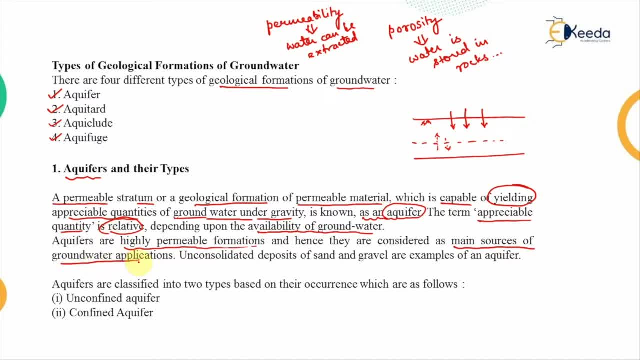 which are in the irrigation and the domestic municipality needs. Now the unconsolidated deposits, that means the deposits of the sand which are not being consolidated, and of the gravel. they are the prime example of an aquifer. Now, depending upon their occurrence, where they are available, 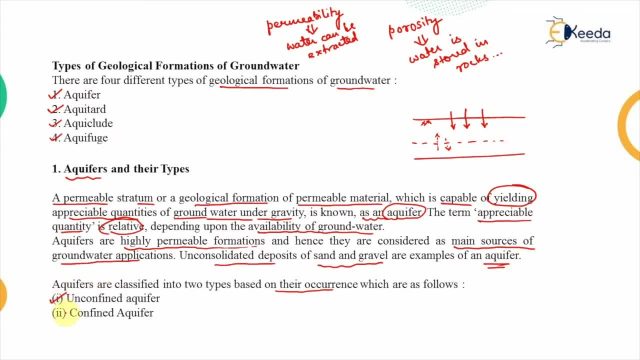 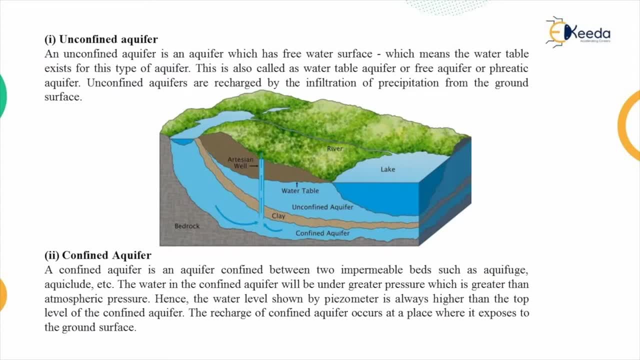 they are classified into two categories: that is the unconfined aquifer and second one is the confined aquifer. Now, the name itself suggests that what is an unconfined one and what is a confined aquifer. So an unconfined aquifer is an aquifer which has free water surface. 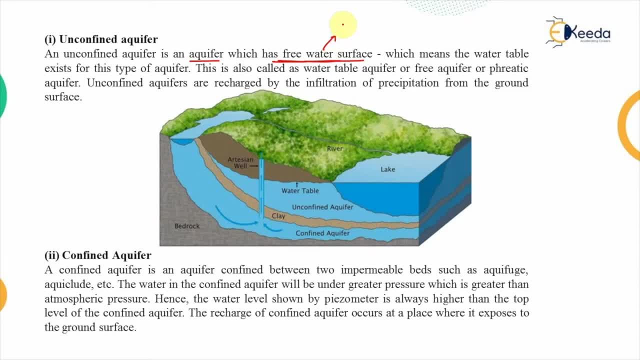 That means there will be no formation or layer above the free water surface. That means the water table exists for this type of aquifer, because water table should have a free surface. This is also called as the water table aquifer or the free aquifer, or the phreatic aquifer. 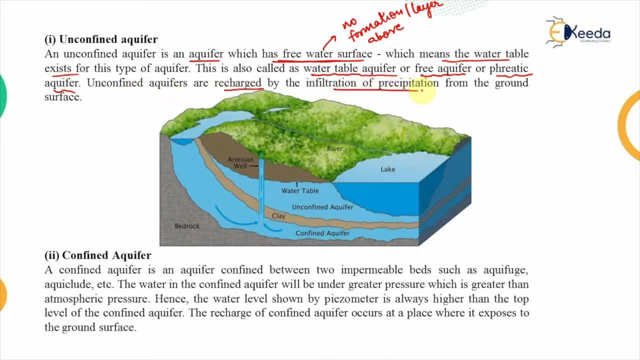 They are recharged by the infiltration of the precipitation, in which the major component is from the rainfall, and they percolate from the ground surface. Now, this unconfined means from one side it will be having certain layer. for example, in this image there is a clay layer, so that's why there will not be any further percolation. 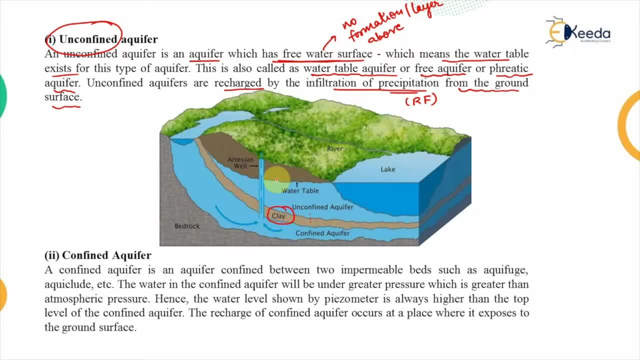 and the top surface is free. So the water table is available up to this particular point. So this aquifer, which is storing the water, is confined from one side and is free from the other side. Such structure is known as the unconfined aquifer. 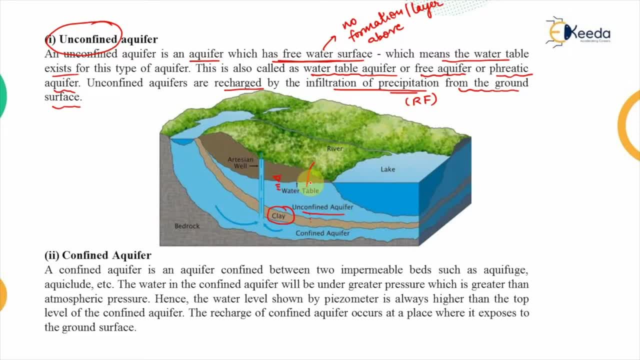 And from here we can extract the water directly with the help of certain lift mechanisms. The second one is the confined aquifer. Now, that means it will be having its boundaries confined within the two layers, So it is an aquifer which is confined between the two impermeable beds, such as aquifuse and aquiclude. 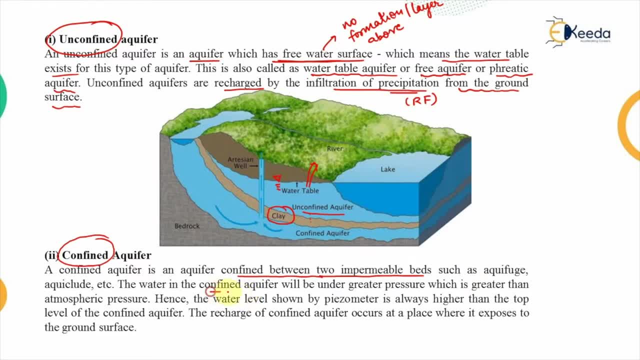 What are these That we will see? The water in the confined aquifer will always be under the greater pressure, which is greater than the atmospheric pressure. Let's say, if this is a water surface which is exposed to the atmosphere, then the pressure which will be applied here, that will be atmospheric pressure. 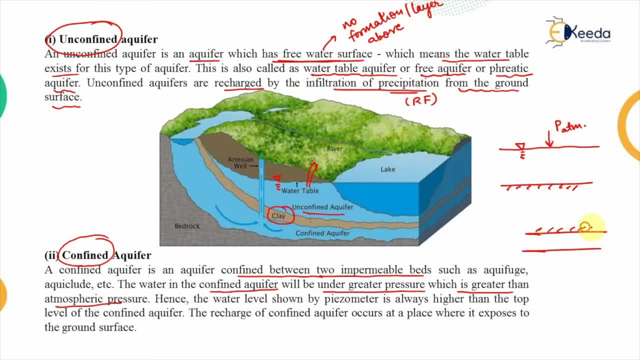 But if there is any closed surface and within this the water is flowing. So the water that will be flowing under certain pressure and that pressure will be greater than the atmospheric pressure. So the water level which will be shown by the piezometer, 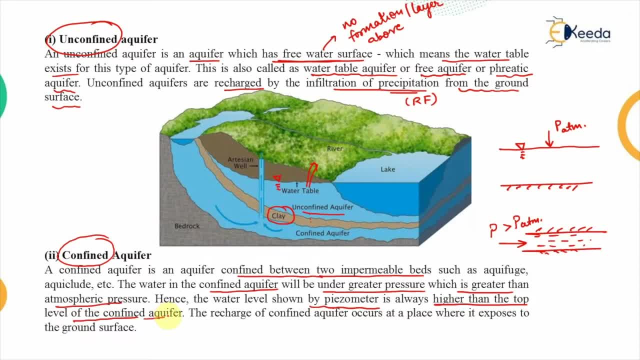 that is higher than the top level of the confined aquifer. Now, the recharge of such structures, that occurs at those places where it is exposed to the ground surface, Because otherwise there is no entry point into these kind of aquifers. So, as you can see in this image, this confined aquifer is sandwiched between the clay layer and this bedrock. 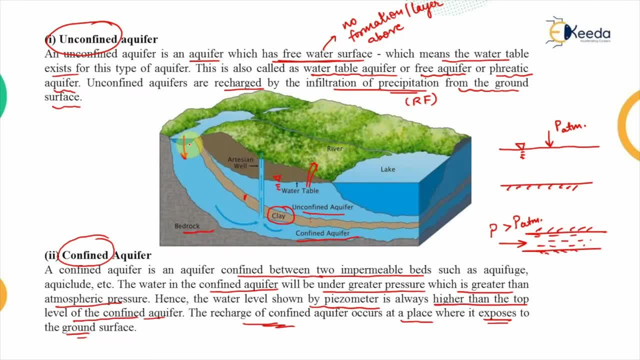 And it is being recharged from the point where it is exposed to the ground surface. And when it is under pressure, then it will be rising through any openings under the piezometric head which is available to it And because of this there will be the formation of the springs that you observe. 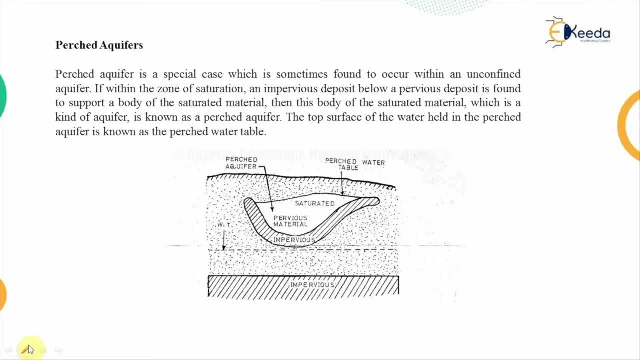 There is one more type of aquifer which is a special case. So it is sometimes found to occur within an unconfined aquifer. So unconfined is the one in which one layer is impervious, other one is free. 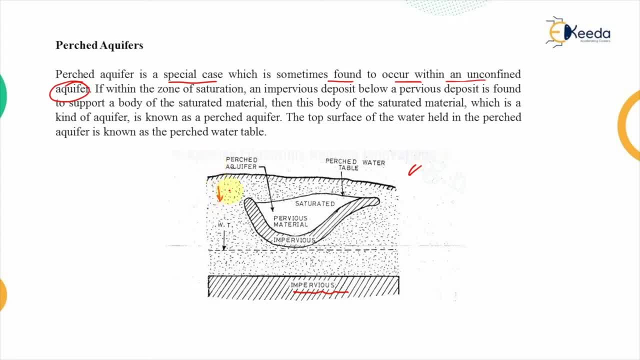 So within this zone of saturation- that means the area where the water is getting percolated- there will be an impervious deposit, below a pervious deposit, which support a body of the saturated material. This kind of aquifer is known as the purged aquifer. 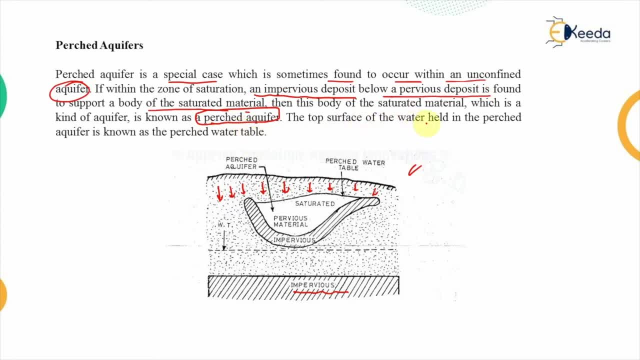 And the top surface of the water held in this purged aquifer is known as the purged water table. So, as you can see, this is a layer which is impervious. Now, the water which will be percolating here, that will be stored on it. 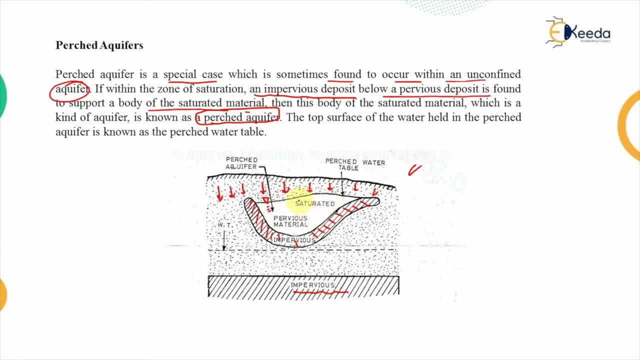 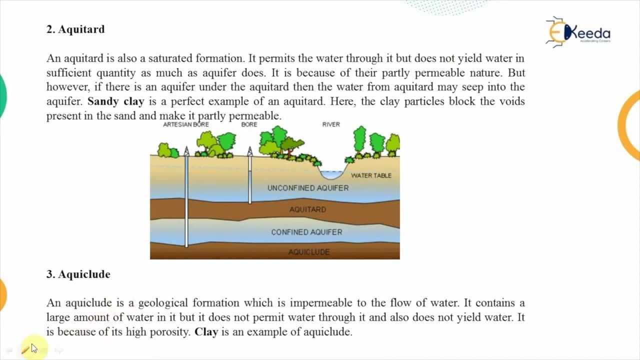 And this type of aquifer, or this type of geological formation which is supporting the storage of ground water, that is known as the purged aquifer, Moving on to the next type of geological formation, that is aquitard. So aquitard is also a saturated formation. 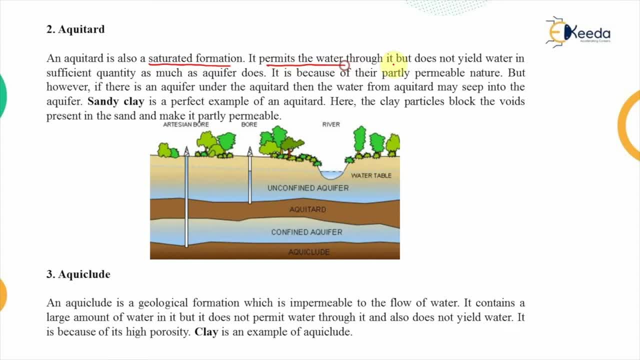 Now what it does? it permits the water through it, but it does not yield the water in sufficient quantity, As much as aquifer does. So that means it is porous, It is allowing the water to flow through it, But it is not yielding the water. 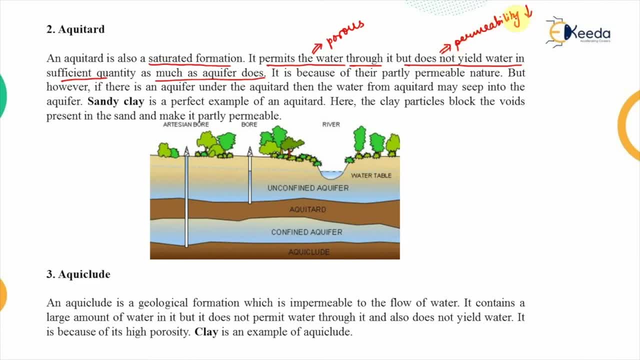 Therefore permeability is less. In this case It is because of their partly permeable nature. That means within this aquitard the water will be stored, but we would not be able to extract the water in sufficient quantities. So if there is any aquifer under the aquitard, 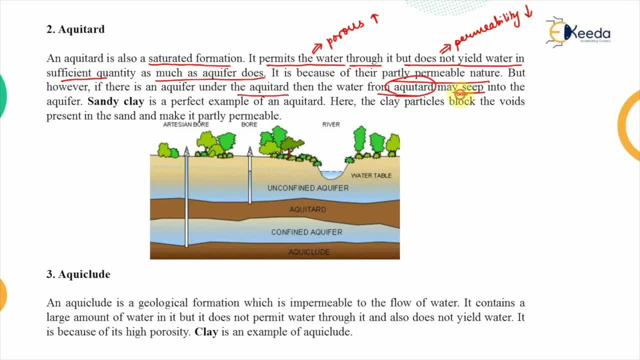 then the water from this aquitard that may seep into the aquifer. The example of it is the sandy clay. Now, if this is the sandy clay, then there will be very less permeability, which will be available, However, since the clay is a fine soil. 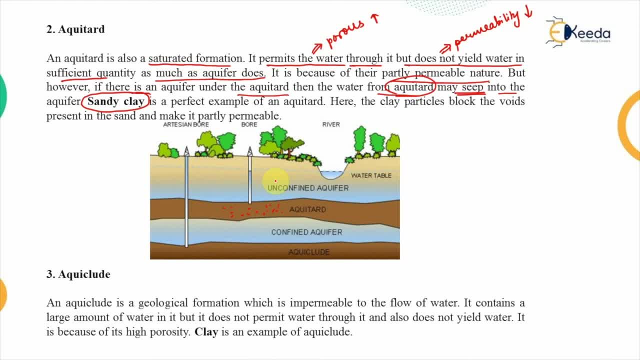 therefore the number of voids. they will be very high And because of which the water will be able to store in this particular soil layer. Now the next formation is known as the aquiclude, So it is a geological formation which is impermeable to the flow of water. 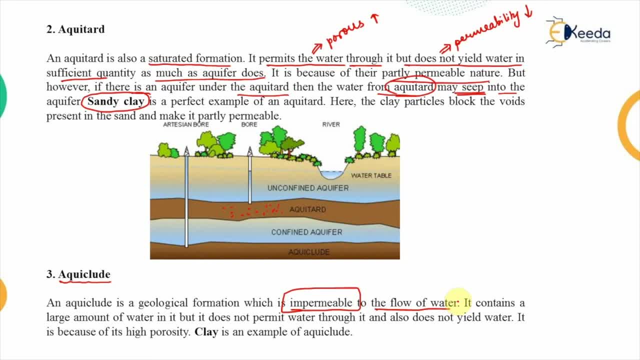 So that means it would not allow any amount of water which can be yielded from it or can be extracted from it. So it contains a large amount of water, but it does not permit the water through it and therefore does not yield any water. 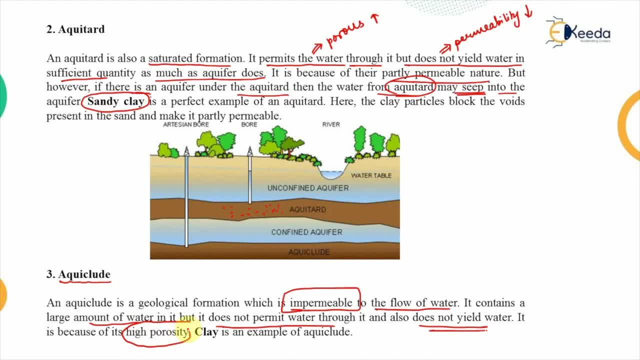 And it is storing the water because of its high porosity. The prime example of it is the clay layer. So this is a clay layer which is forming the bedrock. Then, middle layer, this is the sandy clay. So this sandy clay which is allowing certain portion of the water. 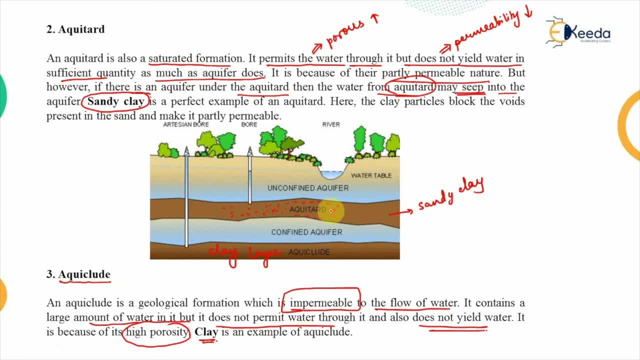 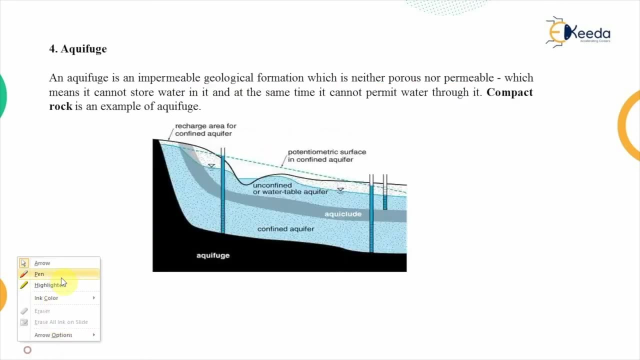 that is aquitard because it is retarding the water speed, the rate at which the water was extracted in case of the aquifer. Therefore, the name comes as the aquitard. The last of the formation is known as the aquifuse. 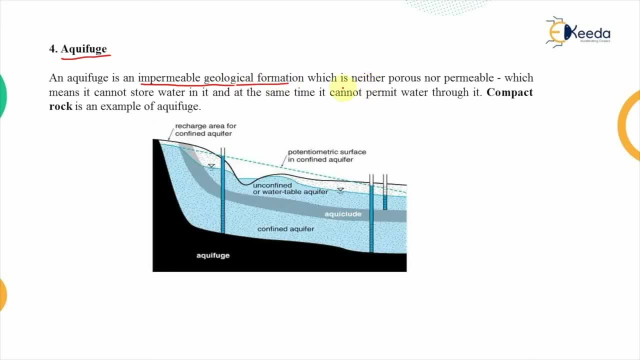 So it is an impermeable geological formation which is neither porous nor permeable. That means if it is not porous, we cannot store the water in it, and if it is not permeable, we cannot extract the water through it. The example of it is the compact rock. 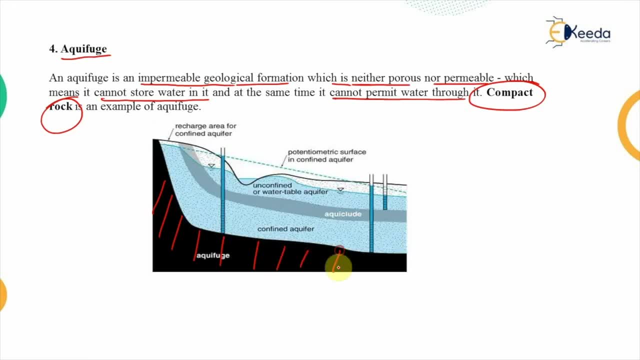 So, as you can see in this image, this black structure, this black portion that is known as the aquifuge, in which neither the water can be stored nor can be extracted out of it. Now, if we look at the next table, this would give us the comparison of the different groundwater formations. 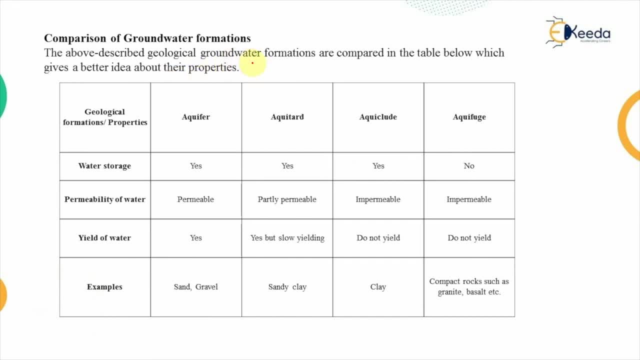 Now all the above described geological groundwater formations are compared in this table To have the better idea. So one by one, this is aquifer, then aquitard, then aquiclude, and last one is the aquifuse. So the first parameter is the water storage. 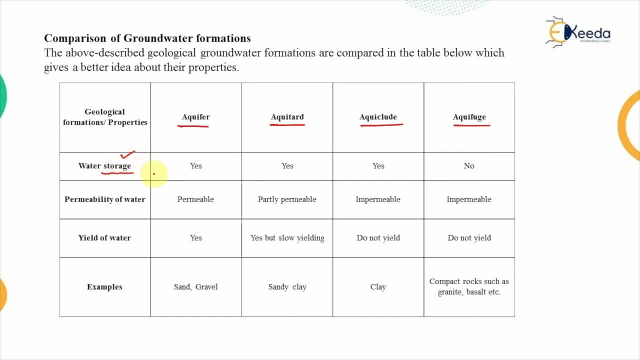 Whether we would be able to store the water in it or not. So in aquifer we can store the water. In aquitard we can store the water. In aquiclude also we can store the water. But in aquifuse there is no storage of the water. 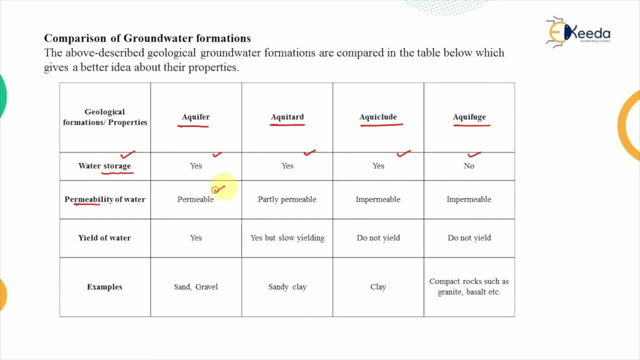 Then permeability. Aquifer is permeable because we can extract the water, Aquitard because it is retarding the extraction rate. Therefore it is partly permeable And aquiclude. this is impermeable. We can store it in it but we cannot extract out of it. 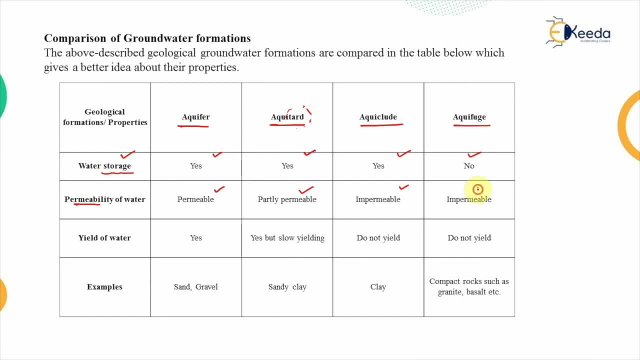 And similarly aquifuse is neither porous nor permeable. Now, this permeability is directly related to the yielding. So if it is permeable, then it is yielding. If it is partly permeable, then it will be a slow yielding.